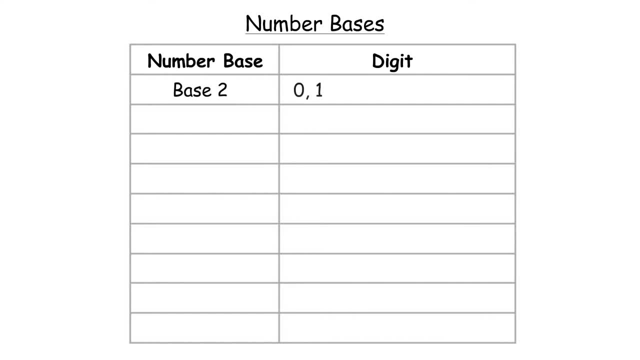 Base 2 will use 2 digits which are 0 and 1.. Base 3 will use 3 digits which are 0, 1 and 2.. Base 4 will use 4 digits which are 0 to 3.. Base 5 will use 5 digits which are 0 to 4.. 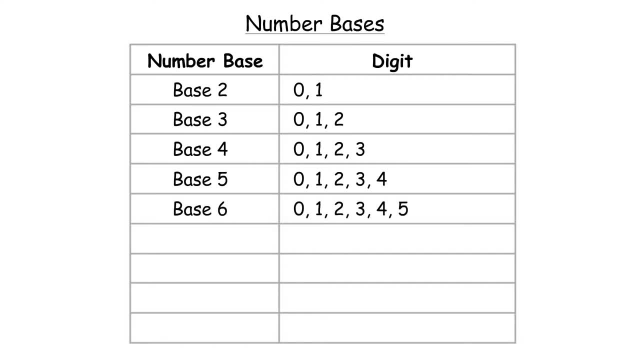 Base 6 will use 6 digits, which are 0 to 5. Follow by Base 7., Base 8., Base 9. And Base 10 will use 10 digits, which are 0 to 9.. For instance, how many balls are there in the following? 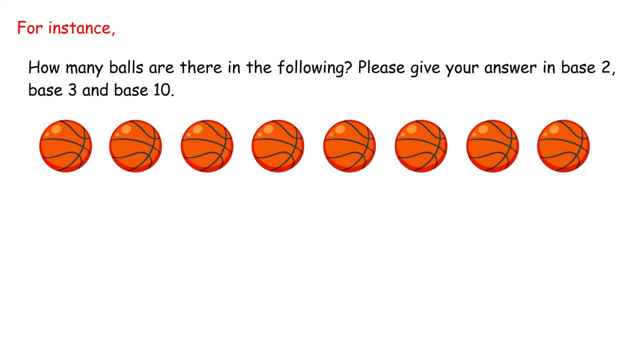 Please give your answer in Base 2,, Base 3 and Base 10.. Base 2 only use 2 digits, which are 0 and 1.. Let us count together First 1, then cannot have 2, so become 1, 0.. 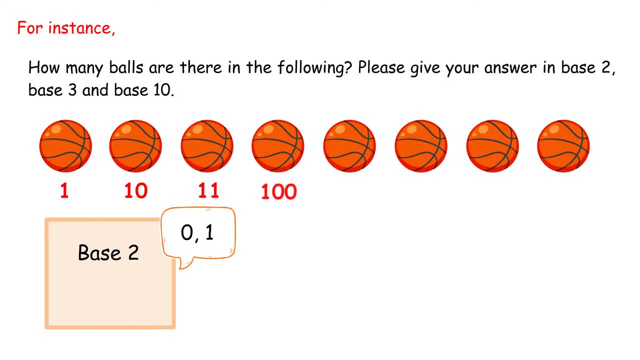 After that: 1, 1.. 1, 0, 0, 1, 0, 1, 1, 1, 0, 1, 1, 0, 1, 11, 10, 1, 0.. 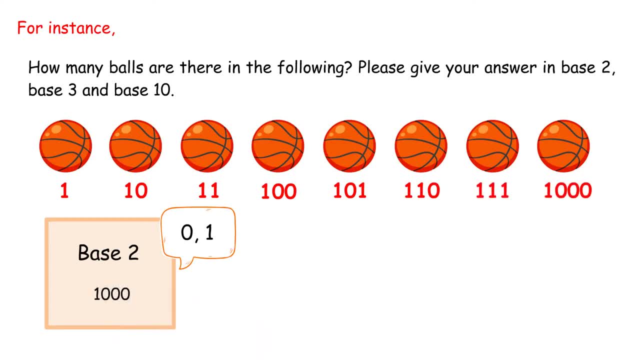 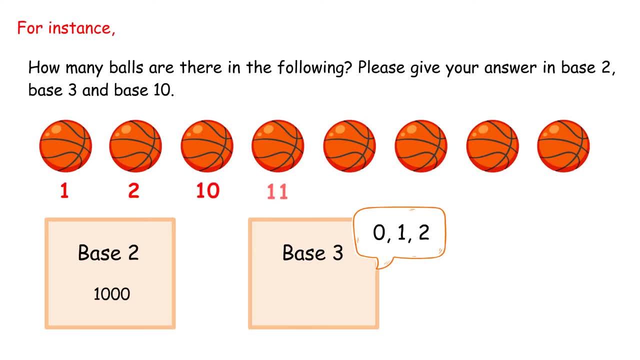 Follow by 2, 1, 0, 1, 1, 1, 2, 2, 0, 2, 1, and, lastly, 2, 2.. 1, 0, 1, 0, 1, 0, 0, 1, 0, 2, 1, 0, 1, 2, 3.. 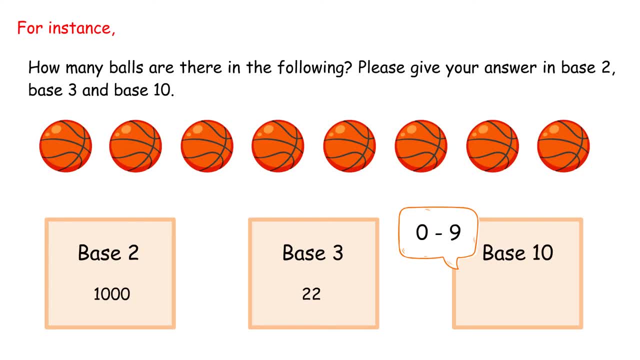 use 10 digits, which are digits from 0 to 9.. First 1,, then 2,, 3,, 4,, 5,, 6,, 7, and lastly 8.. Therefore, the number of ball is 1, 0 0, 0 in base 2,, 2, 2 in base 3, and 8 in base 10.. 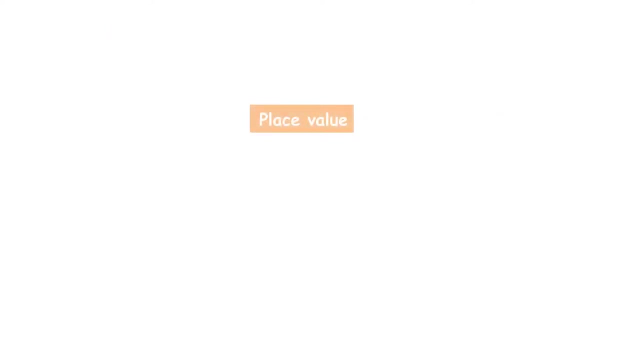 The place values of a base are the repeated multiplication of that base raised to the power of the position number. Example State the place value of each digit in the numbers: A- 6, 2, 3, 1 in base 8.. B- 1- 1, 1, 1, 0, 1 in base 2.. 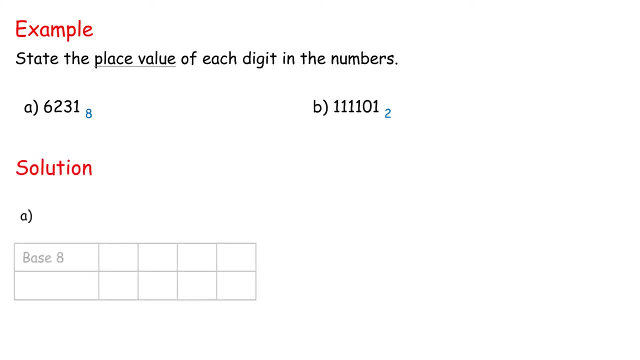 Solution: A: Write down the digit in base 8. 6.. 2, 3, 1.. After that, write down the place value from right to left: A to the power of 0,, A to the power of 1,, A to the power of 2, and A to the power of 3.. 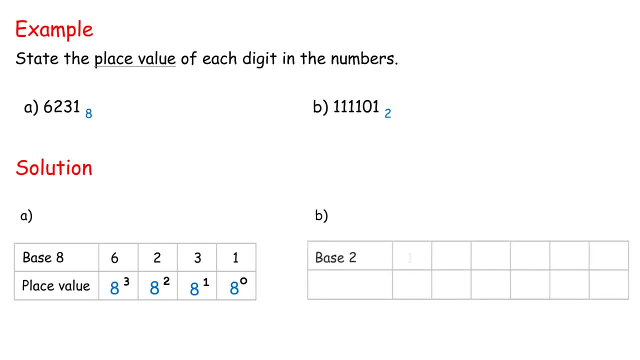 B. Write down the digit in base 2.. 1. 1. 1. 1, 0, 1.. After that, write down the place value from right to left: 2 to the power of 0., 2 to the power of 1,, 2 to the power of 2,, 2 to the power of 3,, 2 to the power of 4, and 2 to the power of 5.. 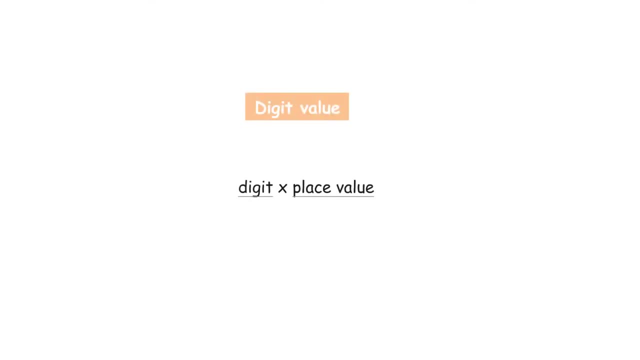 Digit value: The value of a particular digit in the number is the multiplication of a digit and the place value that represents the digit. Example State the digit value of each digit in the numbers A, 6, 2, 3, 1 in base 8.. 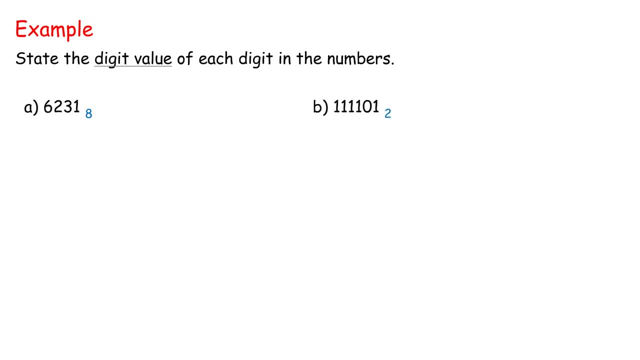 B 1, 1, 1, 1, 0, 1 in base 2.. Solution A: First write down the digit in base 8.. After that, write down the place value from right to left. Next, in order to find out the digit value: digit in base 8, times place value. 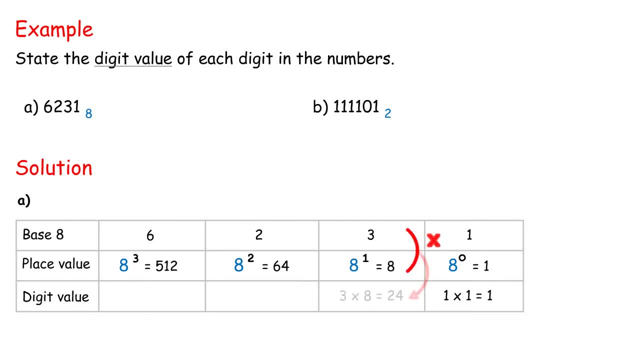 1 times 1 equals 1.. 3 times 8 equals 24.. 2 times 64 equals 128.. And 6 times 512 equals 3072.. B Write down the digit in base 2.. Then write down the place value from right to left. 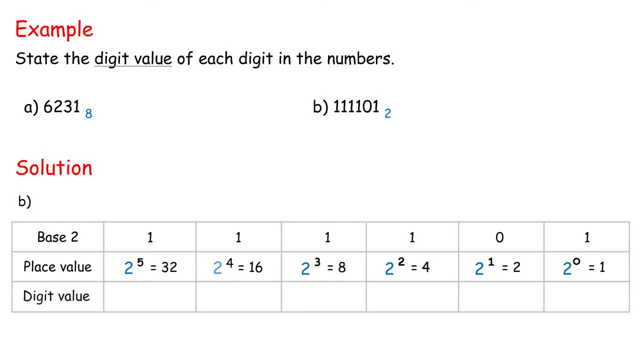 Next, in order to find out the digit value: digit in base, 2, times place value: 1 times 1 equals 1.. 0 times 2 equals 0.. 1 times 4 equals 4.. 1 times 8 equals 8.. 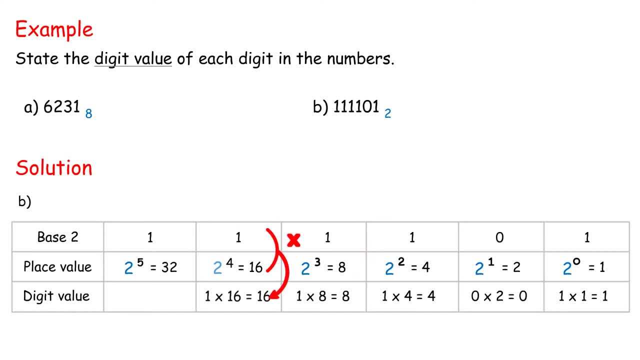 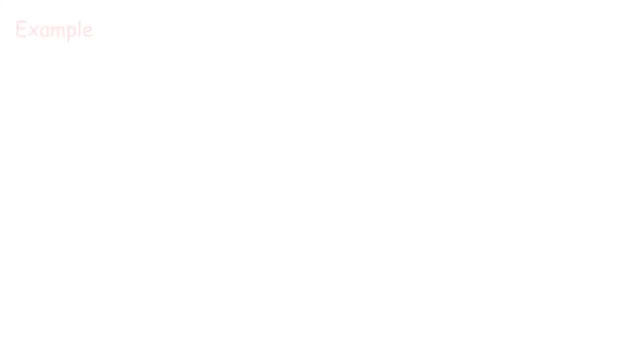 1 times 16 equals 16.. And 1 times 32 equals 32.. Example: State the value of the underlying digit in each of the following numbers: A- 341 in base 8.. B- 5037 in base 9.. 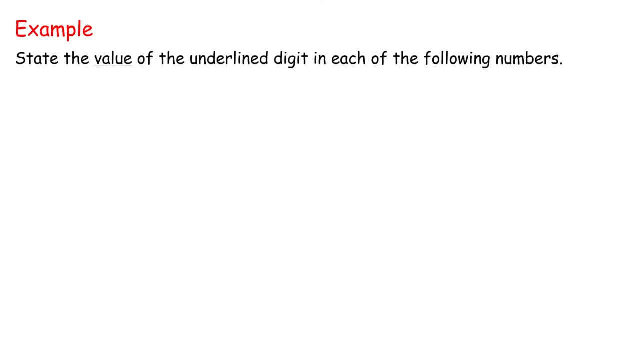 Solution A 341 in base 8.. B 5037 in base 9.. Solution A 341 in base 8.. B 5037 in base 9.. Solution A 341 in base 8.. B 5037 in base 9.. 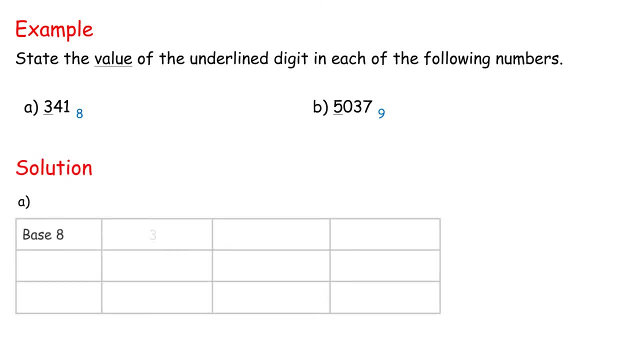 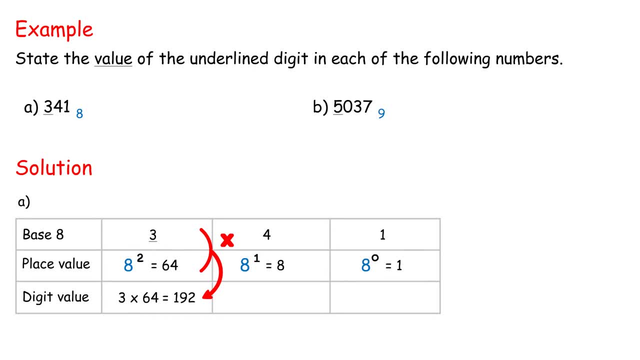 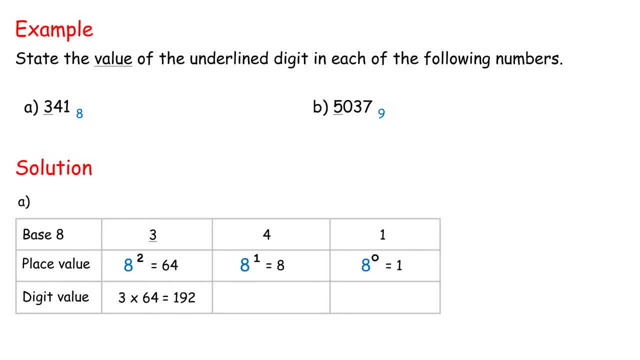 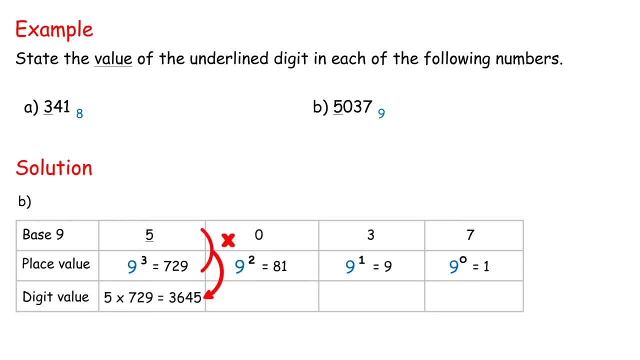 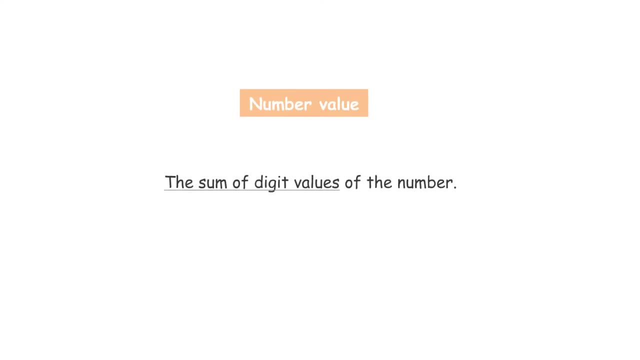 5 times 729 equals 3645. therefore, the value of the underline digit is 3645. number value: the numerical value of a number in various bases can be determined by calculating the sum of digit values of the number. example state: the number value of each digit in the numbers a, 6, 2, 3, 1 in base 8: B: 1: 1, 1, 1, 1 0. 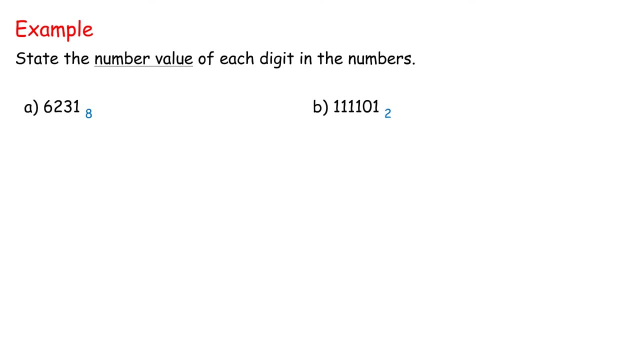 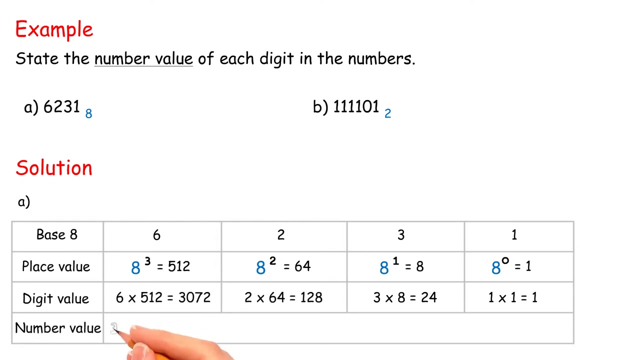 1 in base 2 solution: a: first write down the digit in base 8. after that write down the place value from right to left. next, in order to find out the digit value: digit in base 8 times place value. then the number value is sum of all the digit value: 372 plus 120 plus 24 plus 1. 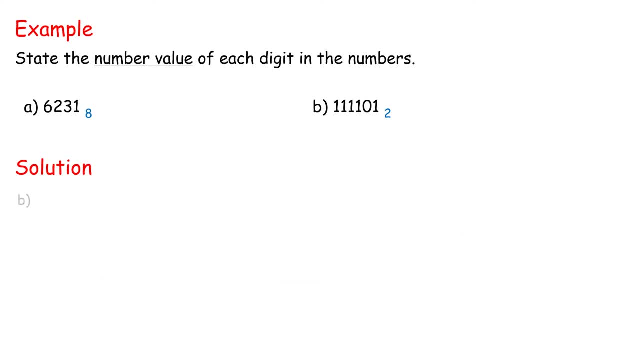 equals 3200, 25 B. first write down the digit in base 2. after that, write down the place value from right to left. next, in order to find out the digit value 2, 2, 5, 1, 2 and 3- opposite- for the ingredients, 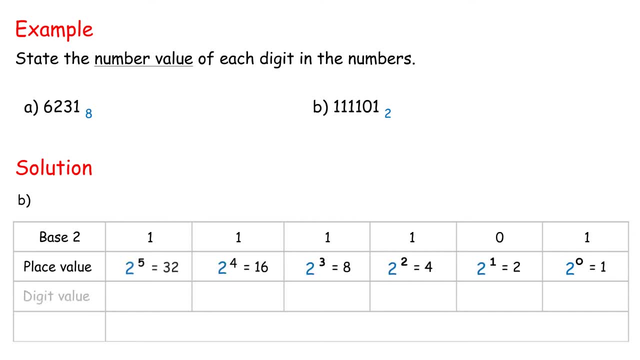 be different. Next, in order to find out the digit value, we need to fix this order. to find out the digit value, digit in base, 2 times place value. then the number value is sum up all the digit value: 32 plus 16 plus 8 plus 4 plus 0 plus 1 equals 61.. after learned the number, 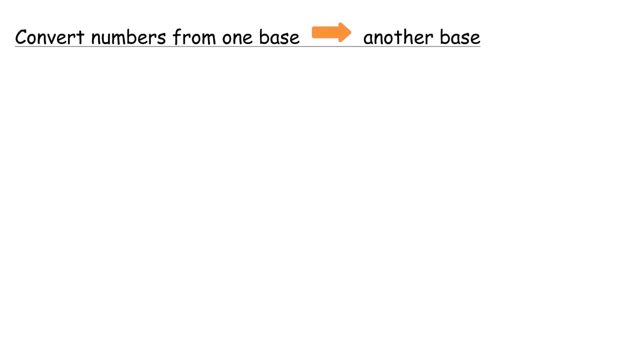 bases. now let us learn how to convert numbers from one base to another base. there are two methods will be discussed here: one, division using place value and two, division using base value. example: rajang river is 563 kilometers. convert 563 in base 10 to a number in a base 5 b, base 8. 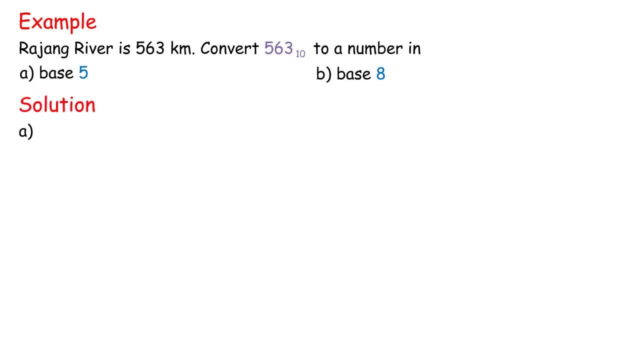 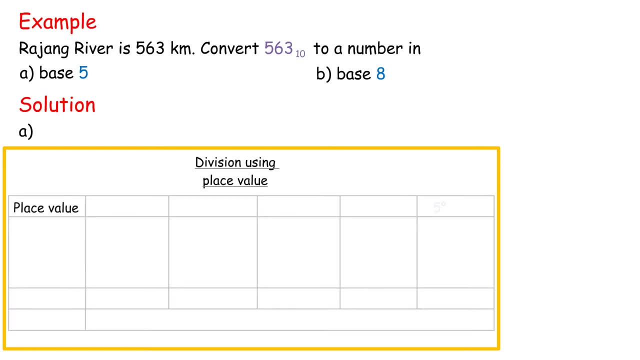 solution: a base 5 method: 1 division using place value. first write down the place value: 5 to the power of 0 equals 1. 5 to the power of 1 equals 5. 5 to the power of 2 equals 25. 5 to the power of 3 equals 125. and. 5 to the power of 4 equals 625. 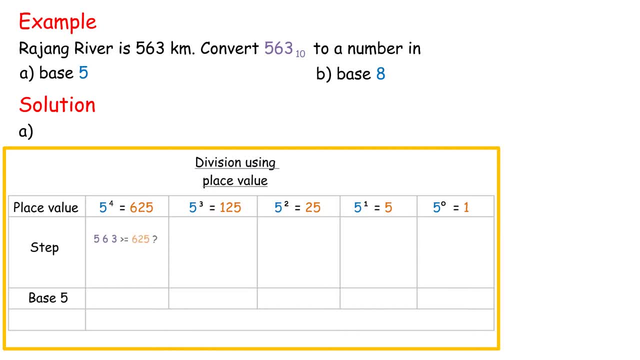 after that, let us check: is 563 greater or equal to 0: 625? no, thus write 0 and base 5. then is 563 greater or equal to 125? yes, thus 563 divide by 125. 4 times 125 equals 500. 563 minus 500 will get 63. 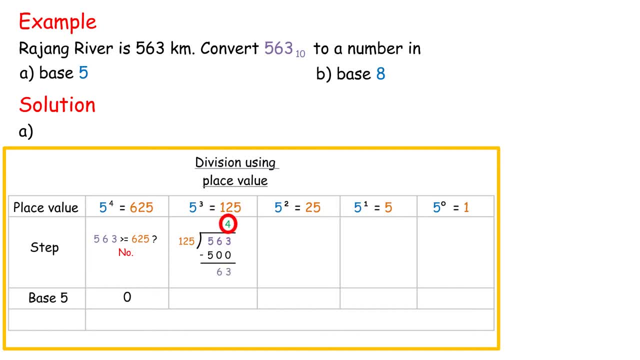 thus write down 4 in base 5, 5 and carry 63 to the next process. is 63 greater or equal to 25? yes, thus 63 divided by 25, 2 times 25, equals 50.. 63 minus 50 will get 13. thus write down 2 and base 13 and carry 13 to the next process. 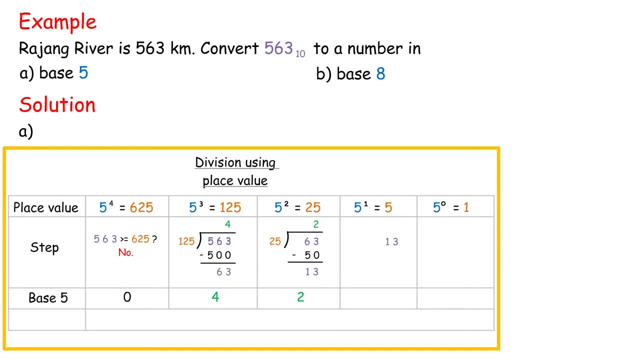 is 13 greater or equal to 5? yes, thus, 13 divided by 5, 2 times 5 equals 10. 13 minus 10 will get 3. thus write down 2 and base 3 and carry 3 to the next process. is 3 greater or equal to 1? yes, 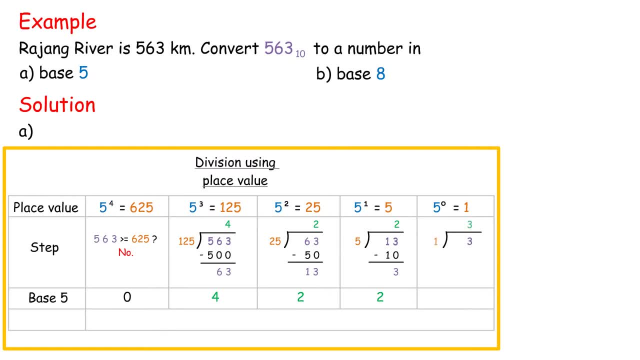 thus: 3 divide by 1, 3 times 1 equals 3,, 3 minus 3 will get 0. Thus write down 3 in base 3.. Therefore 563 in base 10 is equal to 4223 in base 5.. Now let us move on to method 2, division using base value. 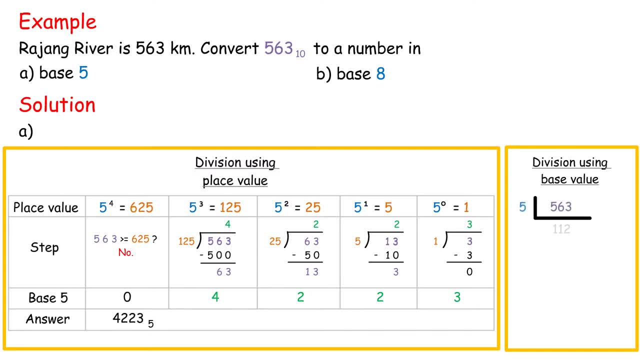 563 divided by 5 will get 112 with the remainder 3.. 112 divided by 5 will get 22 with the remainder 2,. 22 further divided by 5 will get 4 with the remainder 2,. 4 divided by 5 will get 0 with. 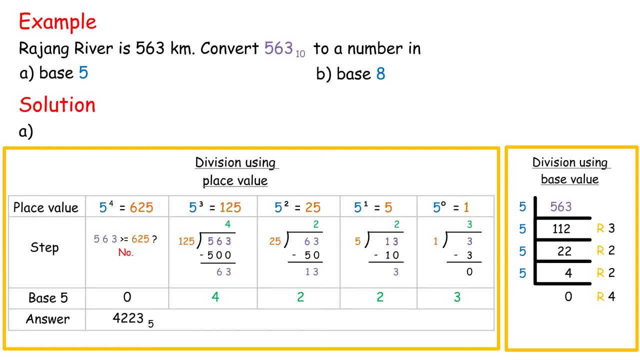 the remainder 4.. After that, get the value of the remainder from bottom to top. Therefore, 563 in base 10, is equal to 4223 in base 5.. You can see. both method will give you the same answer. 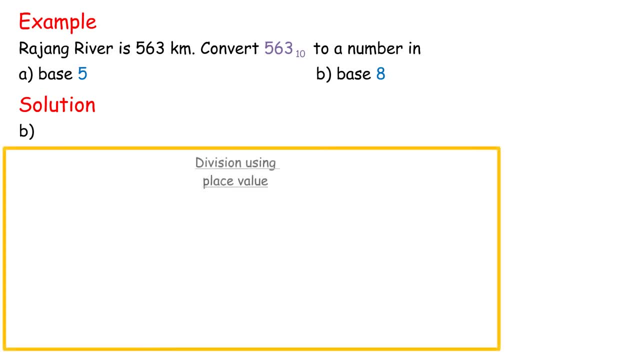 B base 8, method 1, division using place value. First write down the place value: 8 to the power of 0 equals 1,. 8 to the power of 1 equals 8,. 8 to the power of 2 equals 64,. 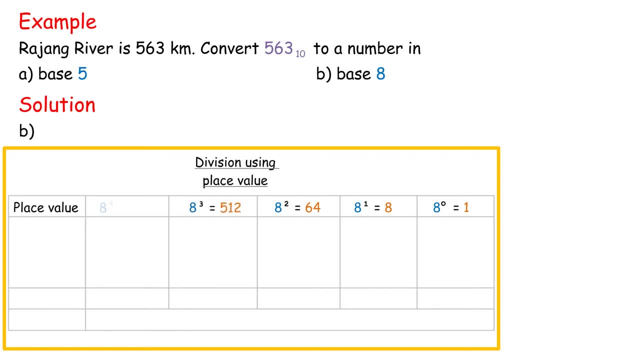 8 to the power of 3 equals 504.. 12. 8 to the power of 4 equals 4096.. After that, let us check: is 563 greater or equal to 4096?? No, Thus write 0 in base 8.. Then, is 563 greater or equal to 512?. 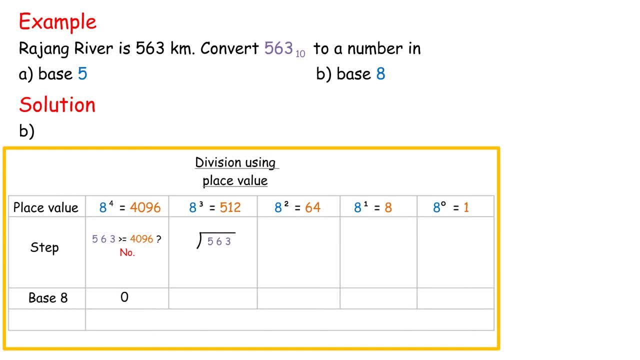 Yes, Thus 563 divide by 512.. 1. times 512 equals 512.. 563 minus 512 will get 51.. Thus write down 1 in base 8 and carry 51 to the next process. Is 51 greater or equal to 64?? No, Thus write 0 in base 8.. Since we never divide, 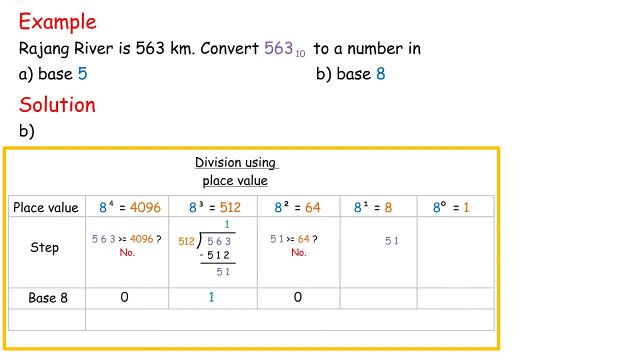 by anything. so carry 51 to the next process. Is 51 greater or equal to 8? Yes, Thus 51 divide by 8.. 6 times 8 equals 48.. 51 minus 48 will get 3.. Thus write down 6 in base 8 and carry 3 to the 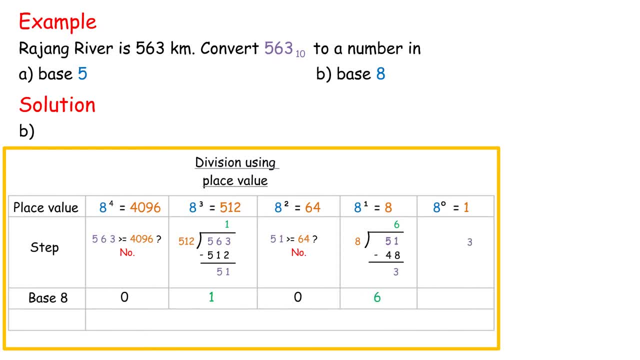 next process: Is 3 greater or equal to 1? Yes. Thus, 3 divide by 1. 3 times 1 equals 3.. 3 minus 3 will get 0. Thus write down 3 in base 8.. 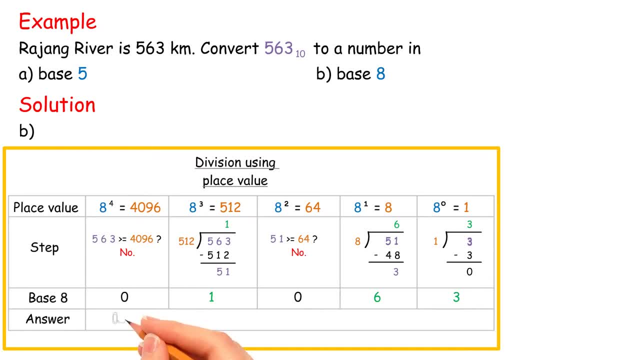 Therefore, 563 in base 10 is equal to 1063 in base 8.. Now we move on to method 2, division using base value: 563 divide by 8 will get 70.. With the remainder 3, 70 divide by 8 will get 8.. With the remainder 6, 8 further divide by 8 will: 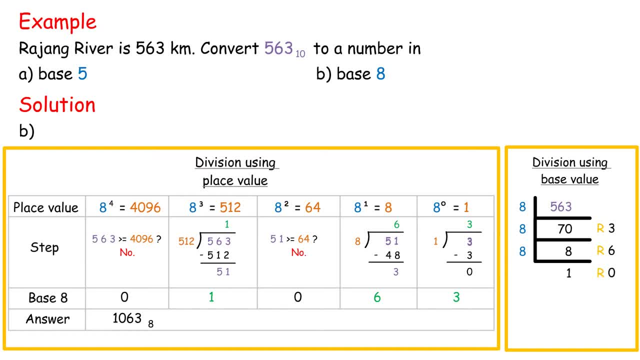 get 1 with the remainder 0. 1 divide by 8 will get 0 with the remainder 1.. After that get the value of the remainder from bottom to top. Therefore, 563 in base 10 is equal to 1063 in base 8.. 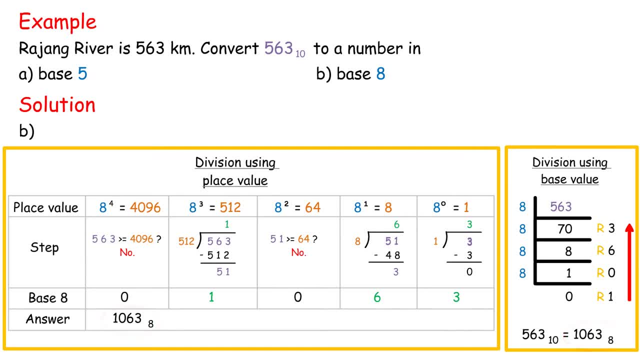 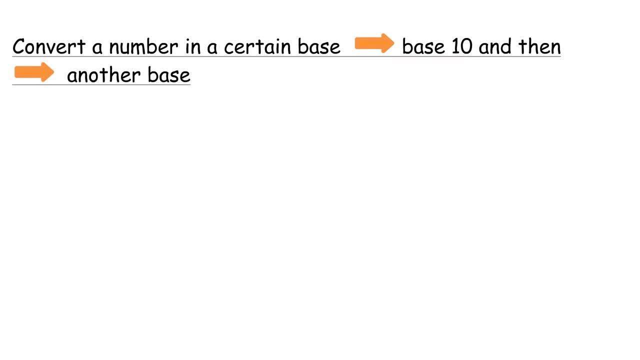 You can see. both method will give you the same answer. Convert a number in a certain base to base 10, and then to another base. A number in base p can be converted to base 10, and then to base q. Example: Convert 253 in base 6 to a number in base 9.. Solution: Step 1. Convert base 6 to 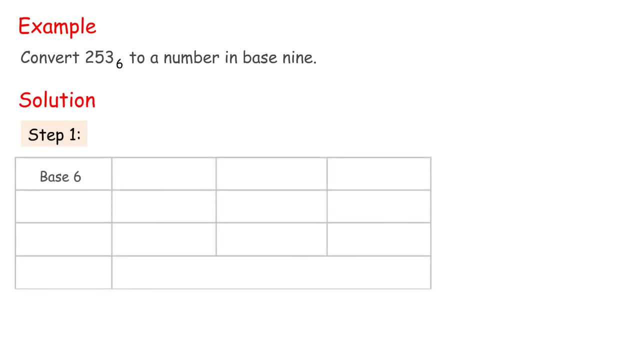 base 10.. First write down the digit in base 6.. After that write down the place value and then count the digit value and lastly add up all the digit value and get the number value. Thus 253. 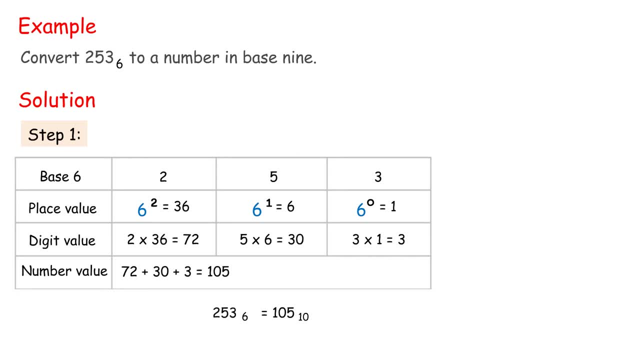 in base 6 equals 105 in base 10.. Step 2. Convert base 10 to base 9.. 105 divide by 9 will get 11, remainder 6,. 11 divide by 9, will get 1, with the remainder 2.. 1 divide by 9, will get 0, with the. 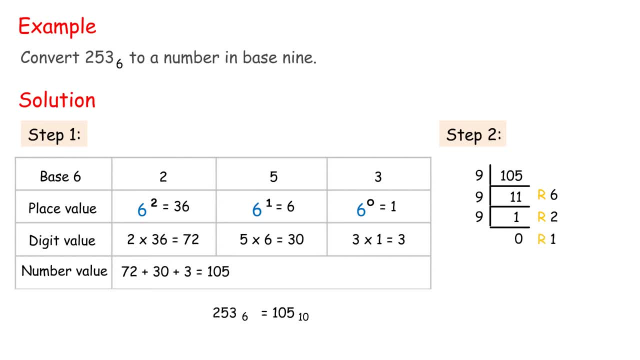 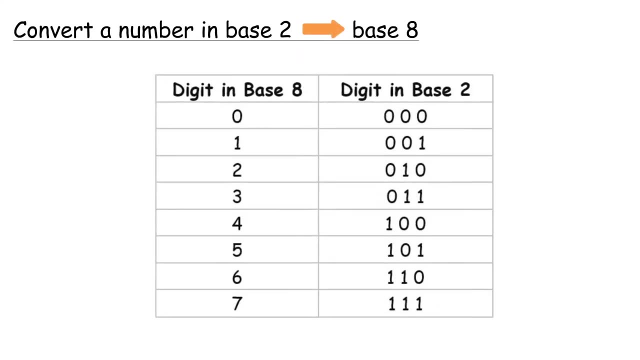 remainder 1.. After that, get the value of the remainder from bottom to top. Therefore, 105 in base 10 is equal to 126 in base 9.. Convert a number in base 2 to base 8.. Each digit in base 8. 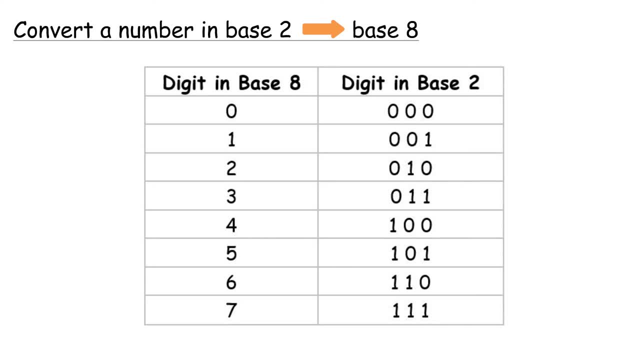 is equivalent to the number in base 9.. Convert a number in base 2 to base 8.. Each digit in base 8 is equivalent to 3 digits in base 2.. Steps 1. Separate each of the 3 digits of a number in base. 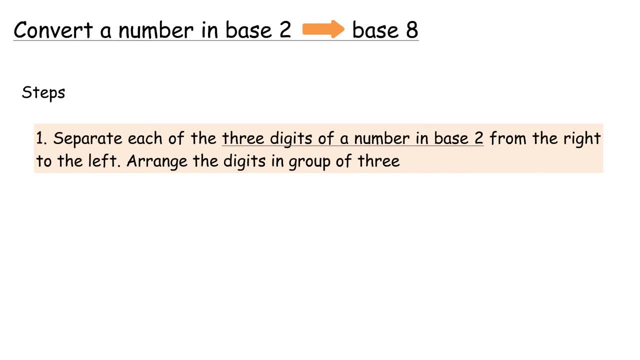 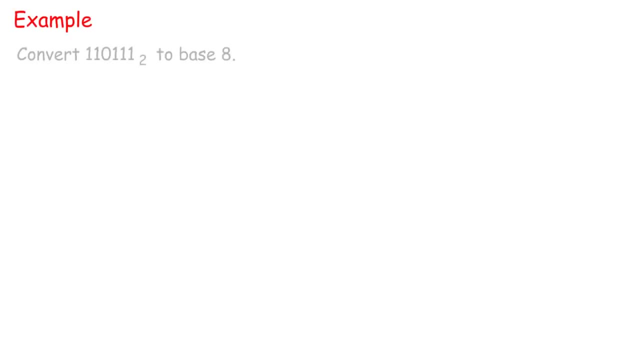 2 from the right to the left. Arrange the digits in group of 3.. 2. Determine the sum of the digit values for the combined 3 digits in base 2.. 3. Combine the number in base 8.. Example: Convert. 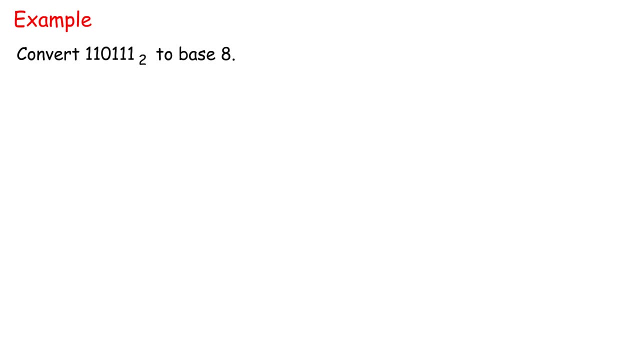 110111 in base 2 to base 8.. Solution: Write down the digit in base 2.. After that write down the place value 3 in one group. Then write down the digit value. Add up the digit value in every group for base 8.. Thus, 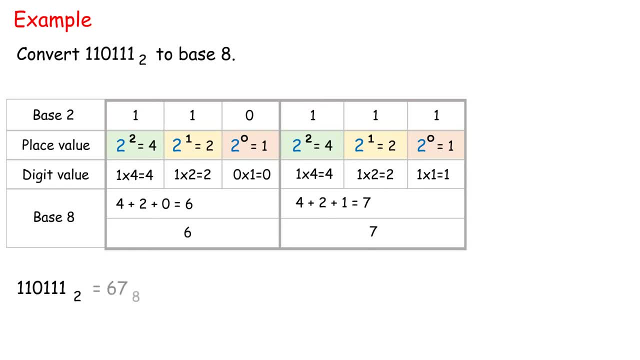 the 110111 in base 2 is 67 in base 8.. The alternative method ways to solve Weiss problem is by listing down the number in base 2 in base 8, and then compare the values. 110 is 6,, 111 is 7,. thus the 110111 in base 2, is 67 in base 8.. Convert a number in base 8 to base 2. 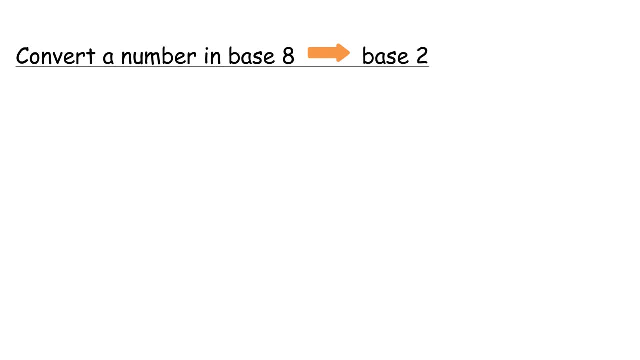 Each digit in base 8 is equivalent to three digits in base 2.. To convert a number 8 to a number in base 2, convert each digit into three digits in base 2 by using 4, 2 & 1. example: convert the numbers in base 8 to numbers in base 2 a. 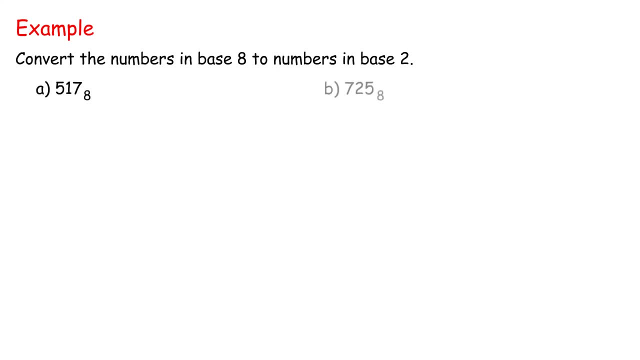 5, 1, 7 in base 8: V 7, 2, 5 in base 8. solution a. write down the digit in base 8: 5, 1 7. 5 is 4 plus 0 plus 1. 1 is 0 plus. 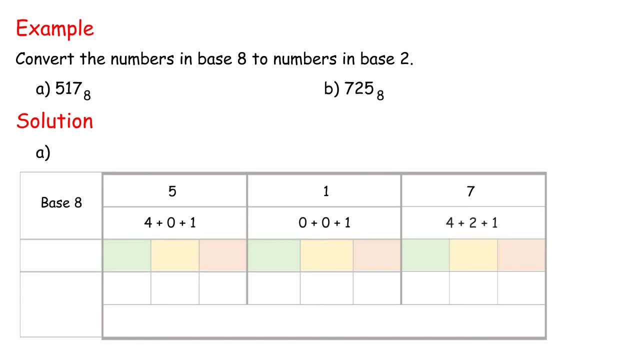 0 plus 1, 7 is 4 plus 2 plus 1. after that write down the place value: 2 to the power of 0 equals 1. 2 to the power of 1 equals 2. 2 to the power of 2 is 4. then 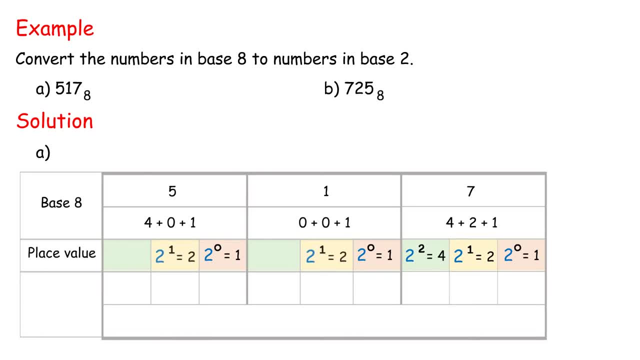 repeat the place value for every group. next write down the digit in base: 2, 5 is 4 plus 1, so below the of the place value of 4 & 1, write 1 and the rest write 0. 1 is 1, so below the. 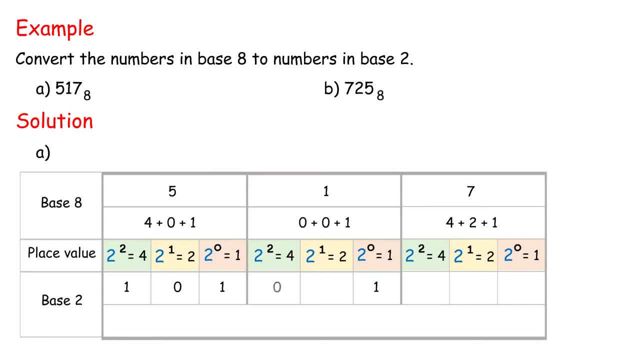 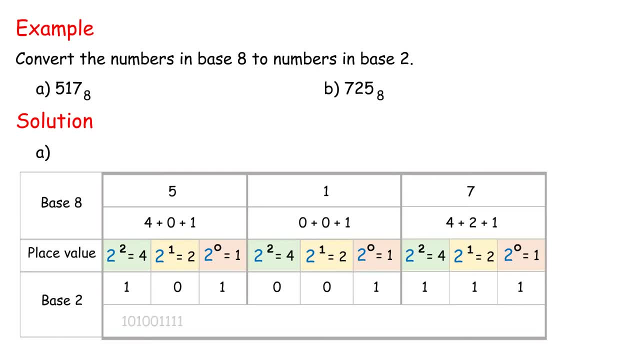 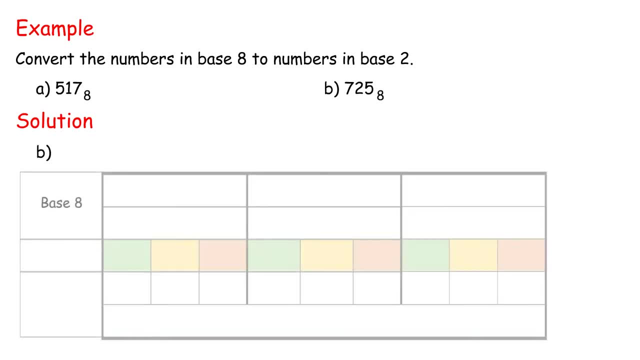 write down the digit in base: 8, 7, 2, 5, 7 is 4 plus 2 plus 1. 2 is 0 plus 2 plus 0, 5 is. write down the digit in base: 8, 7, 2, 5. 7 is 4 plus 2 plus 1. 2 is 0 plus 2 plus 0, 5 is. write down the digit in base: 8, 7, 2, 5. 7 is 4 plus 2 plus 1. 2 is 0 plus 2 plus 0. 5 is 4 plus 0 plus 1. after that, 4 plus 0 plus 1. after, that: 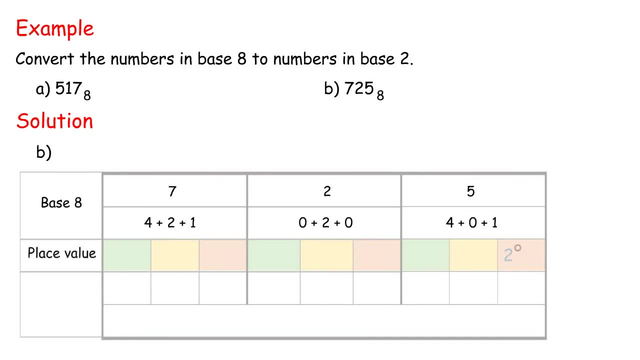 4 plus 0 plus 1. after that write down the place value: 2 to the power of 0 equals 1,. 2 to the power of 1 equals 2,. 2 to the power of 2 is 4, then repeat the place value for. 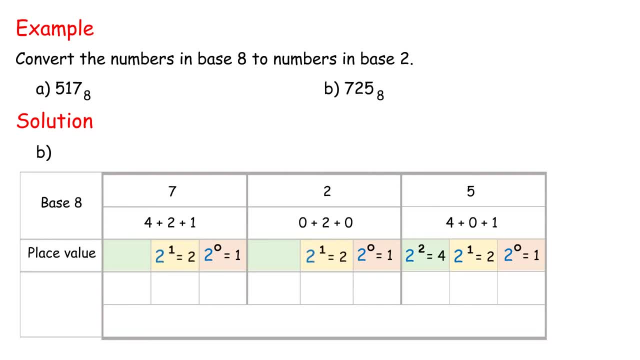 every group. Next write down the digit in base 2.. 7 is 4 plus 2 plus 1,, so below the of the place value of 4,. 2 and 1, write 1, and the rest write 0.. 2 is 2,, so below the of the place value of 2,. 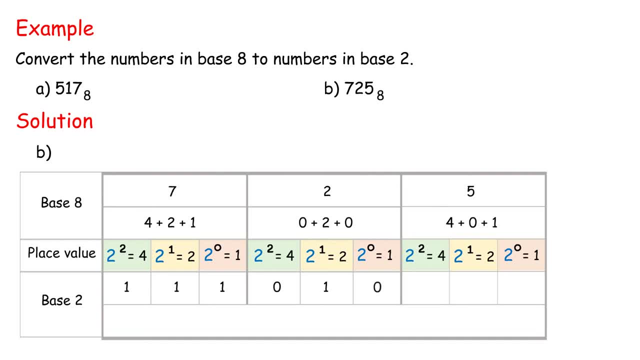 write 1, and the rest write 0.. 5 is 4 plus 1,, so below the of the place value of 4 and 1, write 1.. Therefore, 7 to 5 in base 8 equals 1, 1, 1, 0, 1, 0, 1, 0, 1 in base 2.. 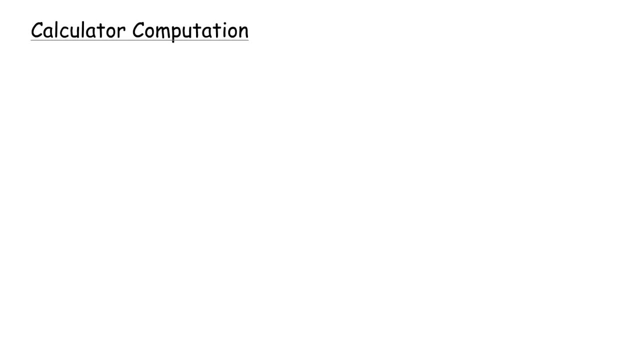 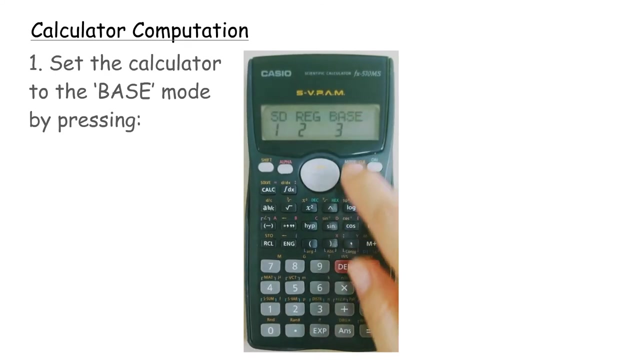 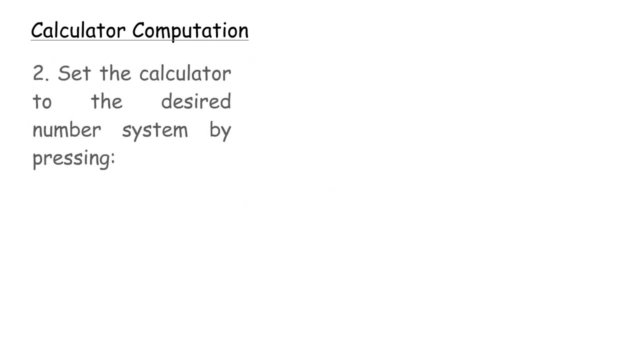 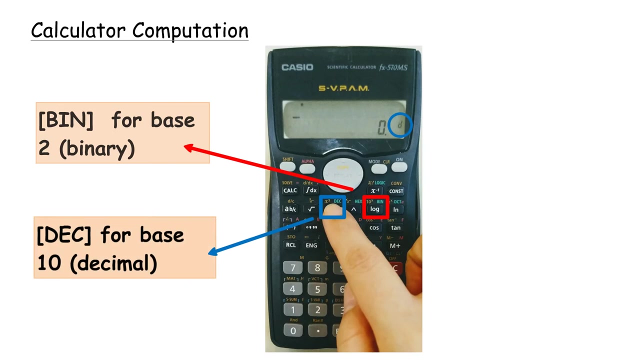 Now let us learn how to use calculator to convert number bases Calculator computation. 1. Set the calculator to the base mode by pressing: 2. Set the calculator to the desired number system by pressing: bin for base 2 binary, dec for base 10 decimal oct. for base 8: octal. 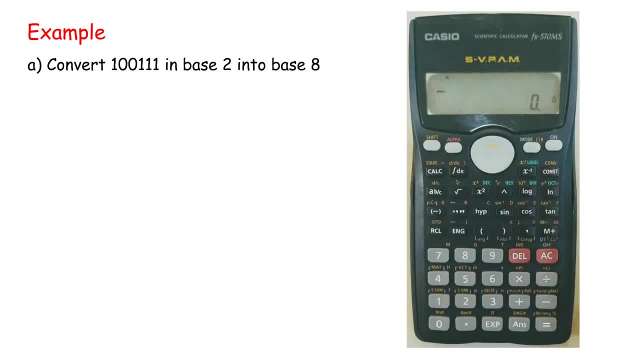 Example A: Convert 1 0 0, 1, 1, 1 in base 2 into base 8.. Therefore, 1 0 0, 1, 1, 1 in base 2 equals 4, 7 in base 8.. 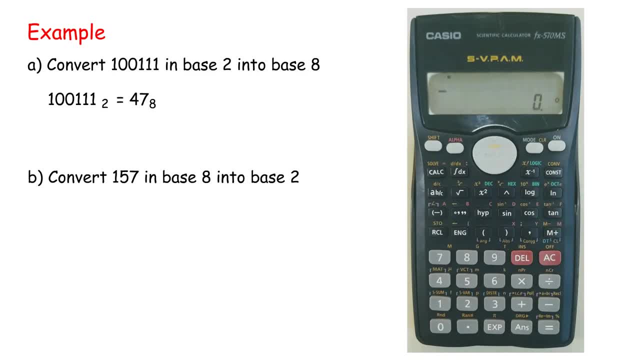 B. Convert 1 5 7 in base 8 into base 2.. Therefore, 1 5 7 in base 8 equals 1 1 0. 1 1 1 1 in base 2.. Addition and subtraction in number bases using two methods. 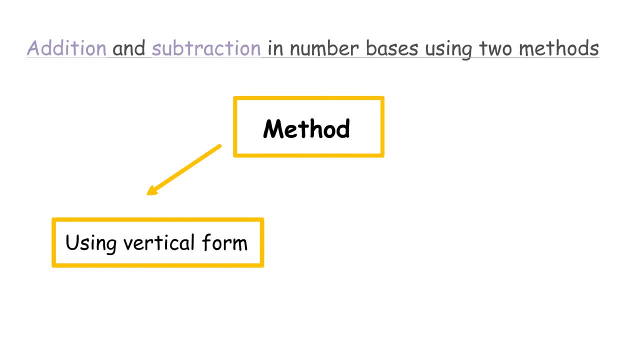 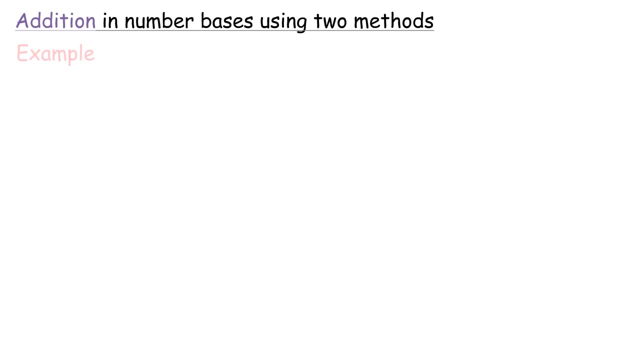 A- Using vertical form: Write the numbers vertically when performing addition and subtraction. B- Conversion of base: Convert the numbers in certain base to base 10.. Addition and number bases: Convert the numbers in certain base to base 10.. Number bases using two methods. Example: Calculate each of the following: A- 1, 1, 0 in base 2 plus 1, 1, 1 in base 2.. 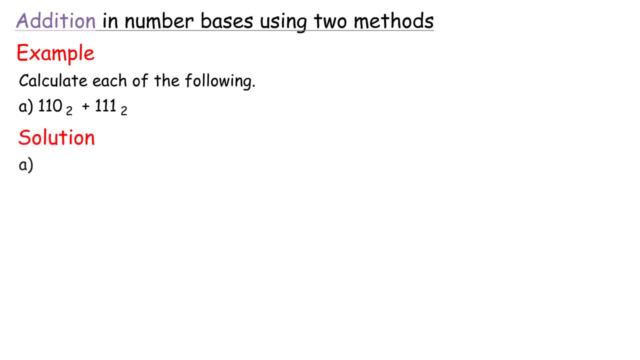 Solution A: E using method 1, using vertical form: 1, 1, 0 plus 1, 1, 1.. 0 plus 1 is 1.. 1 plus 1 is 1, 0.. 1 plus 1 is 1, 0.. 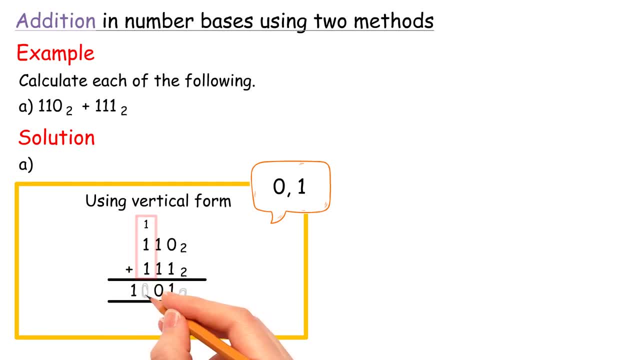 1, 0 plus 1 is 1, 1.. Therefore, the answer is 1, 1, 0, 1 in base 2.. Using method 2, conversion of base: Convert to base 10.. 1, 1, 0 in base 2 is 6 in base 10.. 1, 1, 1 in base 2 is 7 in base 10.. 6 plus 7 equals 13 in base 10.. 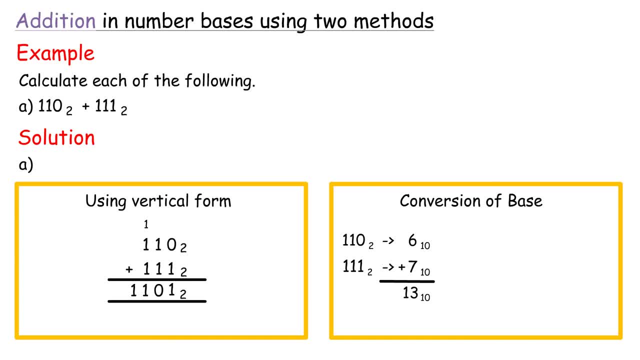 After add up in base 10, we need to convert back to base 13. divide by 2, we'll get 6, with the remainder 1.. 6. divide by 2, we'll get 3, with the remainder 0.. 3. divide by 2, we'll get 1, with the remainder 1.. 1. divide by 2, we'll get 0, with the remainder 1.. 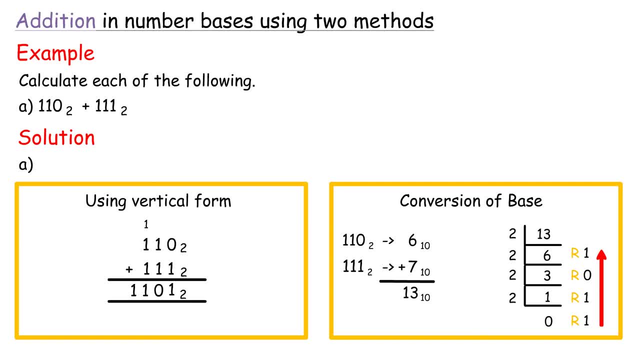 Then get the answer from bottom to top: 1, 1, 0 plus 1, 1, 1 equals 1, 1, 0, 1 in base 2.. You can see. both answers are also the same. 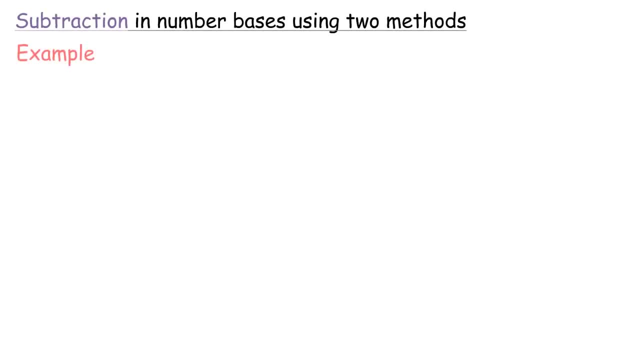 Subtraction and number bases using two methods. Example: Calculate each of the following: A 4, 0, 0, 5 in base 6, minus 3, 2, 5 in base 6.. Solution. 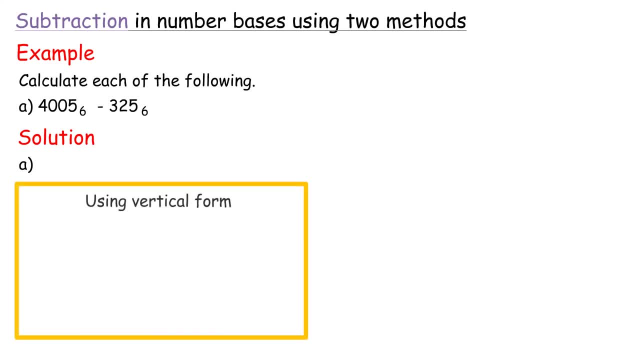 A E. using method 1, using vertical form: 4, 0, 0, 5 in base 6.. 6, minus 3, 2, 5 in base 6.. 5, minus 5 is 0..